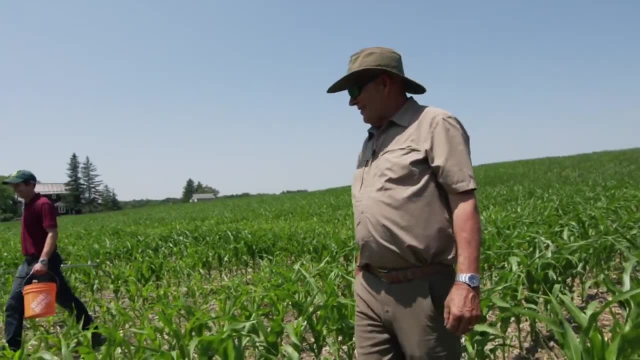 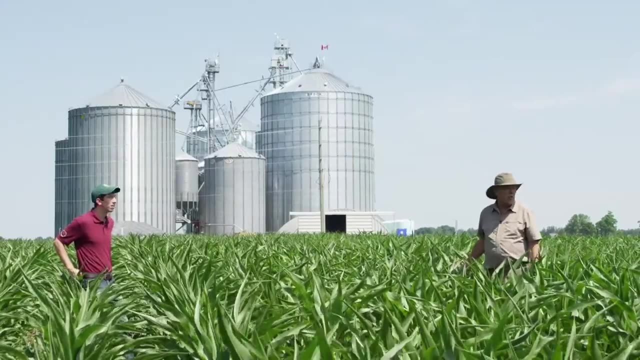 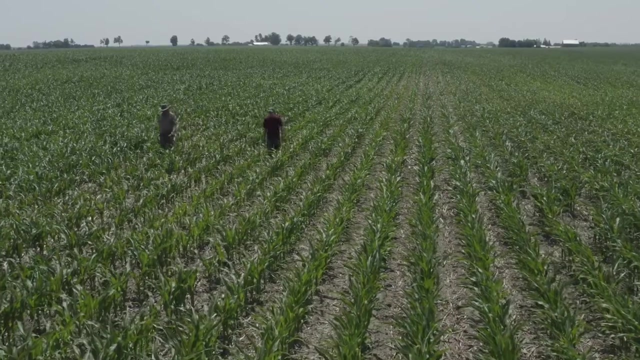 raising the bar on productivity. We have sandy loam or loam ground on this area. We have, as you can see, we have, lots of rolling land, Our family farms in that six, seven thousand acre range of land. We got into soil remediation when we got yield mapping technology back 20 some years ago. 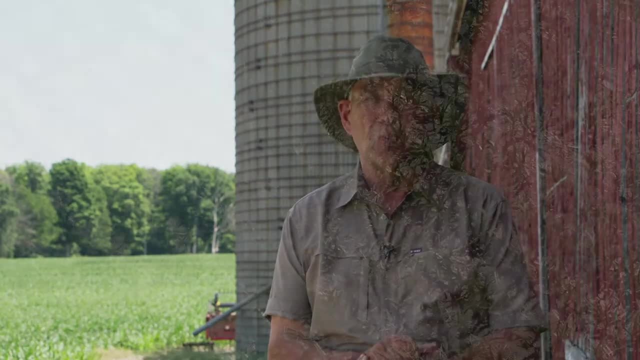 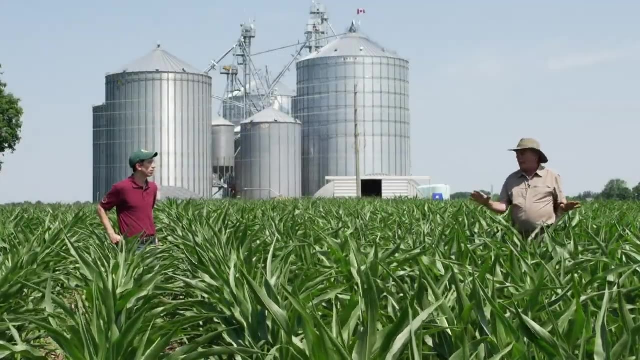 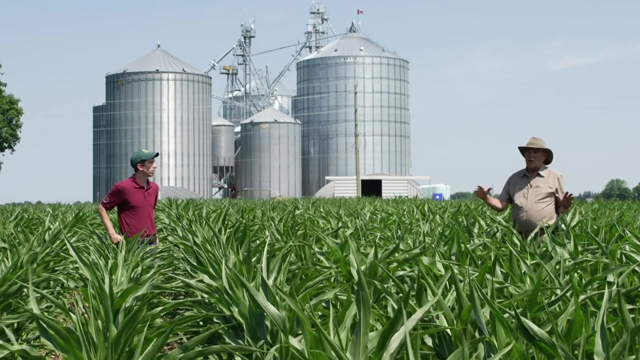 when we came to the shocking reality, The big variation of yield within the field. We tile, drained a lot more ground Places with tough perennial weeds. we went back in to fix those areas up And we also came to realize very quickly that no topsoil means no crop. 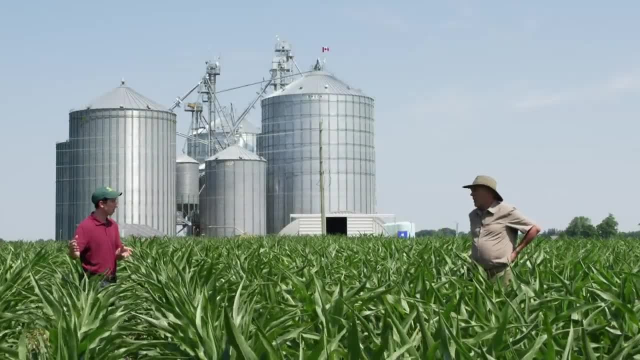 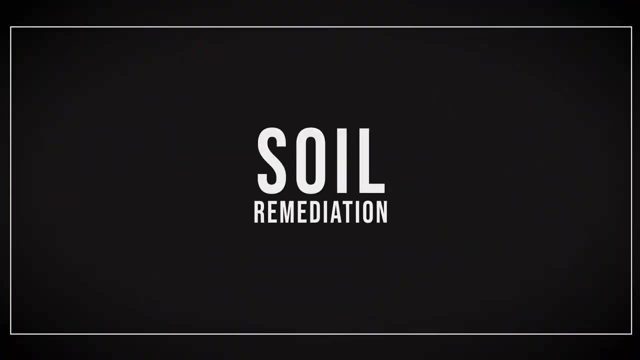 You are taking topsoil from lower slope positions and moving it up to knolls where the topsoil historically has been And lost due to erosion. We use a scraper to take a small amount of soil out of a rich valley, transfer it to. 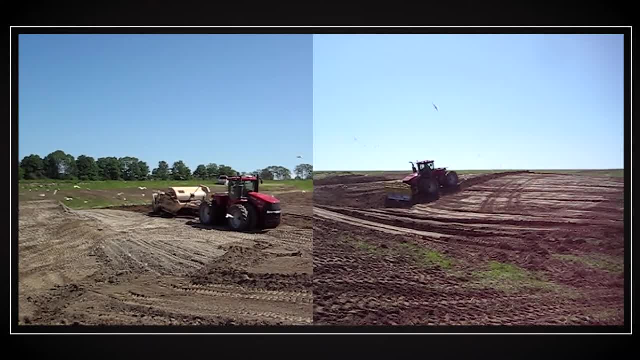 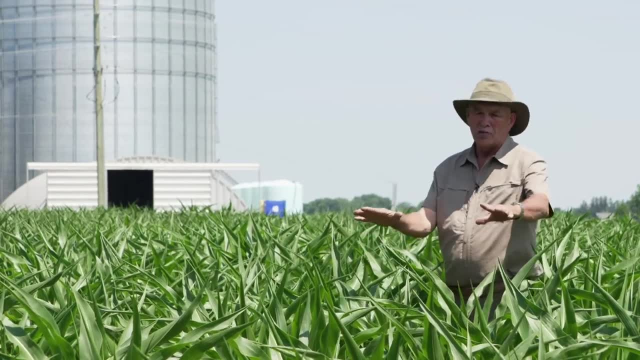 the knoll and a scraper. most scrapers can distribute as they go. Not everybody can have a scraper like what we have now. but you know you could do your own little experiment with a half a day with a front end loader You could. you could cover a nice little knoll. 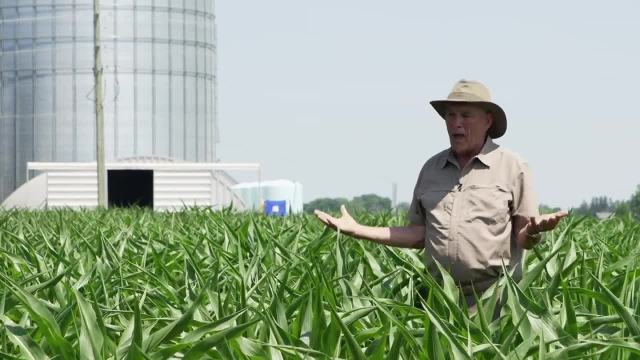 with some dirt. And if you're mapping, or even if you're not mapping, you could. you will see the difference. If you're a tillage guy and the knoll is a little bit bigger, you could cover a nice little knoll with some dirt. And if you're mapping- or even if you're not mapping, you could. you will see the difference. 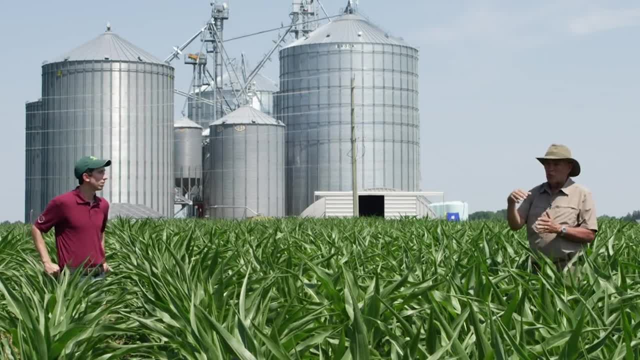 If you're a tillage guy and the knoll is getting less and less, you're losing topsoil. When you till that, you're diluting your topsoil with subsoil. Subsoil is much more erodible. 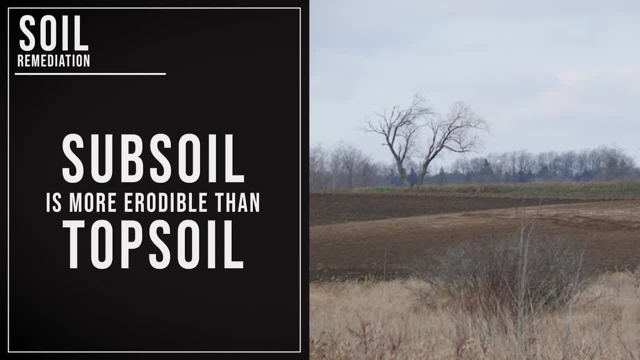 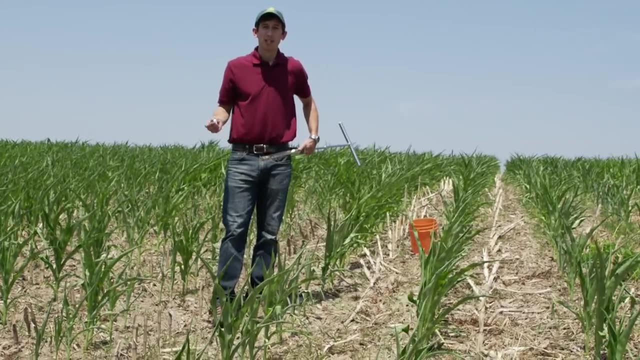 than topsoil. So as you till that hill, or it becomes bare of topsoil, it just becomes more and more erodible because of the nature of topsoil versus subsoil. We're here on a field that has not been remediated, So we've got there's a history of both tillage. 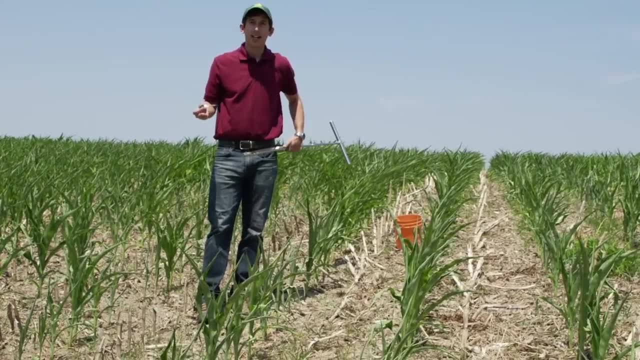 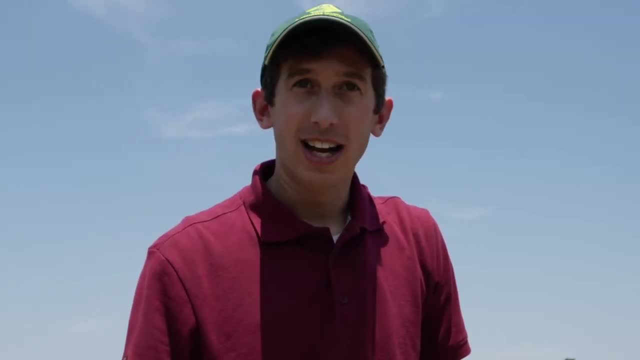 and water erosion And you can see here on July 2nd, the corn is suffering. in this spot There's noticeably more drought stress. One way to evaluate whether you've got parent material mixed in with your topsoil or potentially the topsoil has been completely stripped off of a knoll is to use dilute hydrochloric acid.